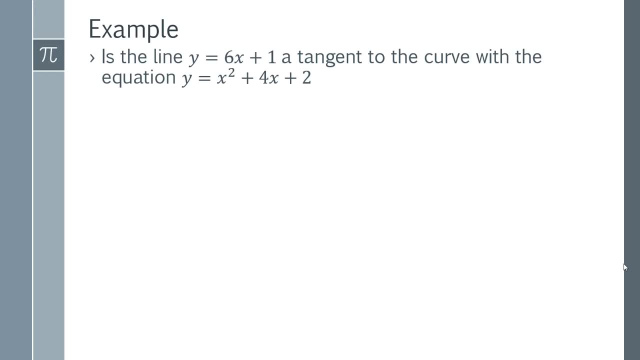 practice. So the question is: is the line y equals six x plus one a tangent to the curve with equation y equals x squared plus four, x plus two, And so we start with our y equals y, and this is very simple. we just set our equation here equal to our equation here, So we're saying that those two 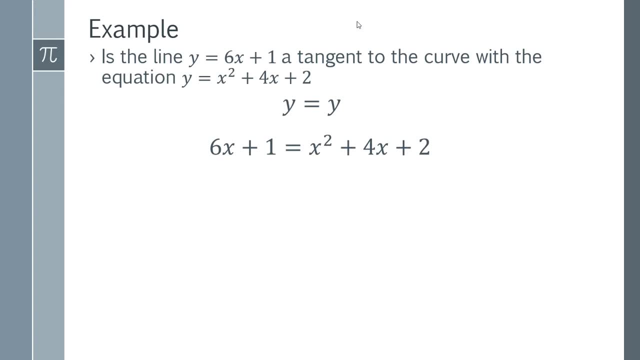 must be equal at one y value and we're going to set our equation here equal to our equation here. So we get that expression. that's just setting the two things equal to each other. We do a simple rearrangement to get an equation equal to zero. You must get equal to zero because you're not. 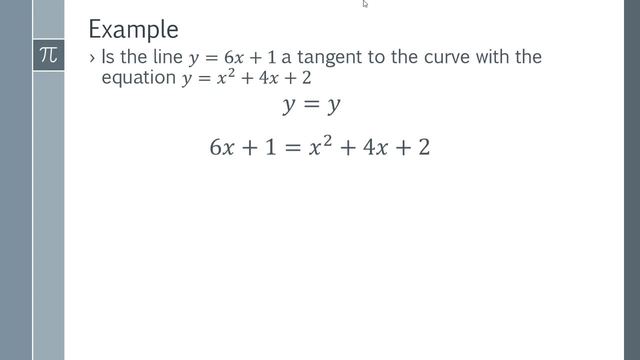 going to be able to use your quadratic formula discriminant, without having equals zero. It doesn't work. So we've got the six x. we'll subtract that to the other side and so that plus four will reduce to a minus two term, and this plus one. we're going to subtract one from both sides and that plus two. 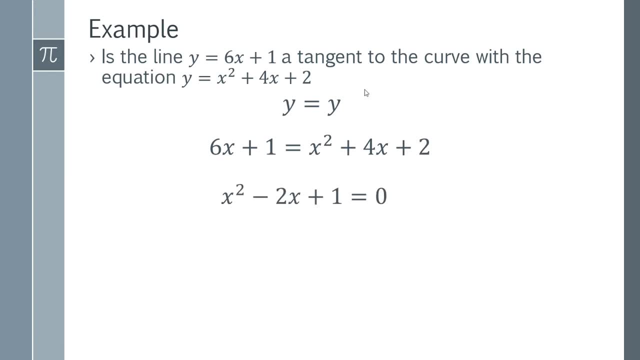 is going to become a plus one. So we end up with that. That's simply rearranging that equation to get equals zero. Our next step is to compare that to the general equation. So we've got ax squared plus bx plus c. That is the. 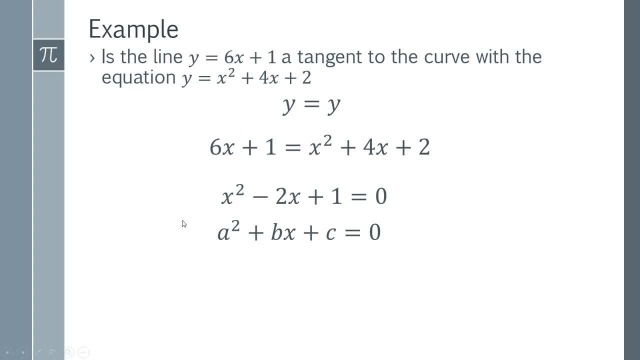 general equation for any quadratic and we can simply compare coefficients. So we've got no number there. so that's telling us that a is going to be one. We've got a minus two in front of the x, so b is going to be minus two. We've got a plus one, so plus c is going to be plus one. So we can. 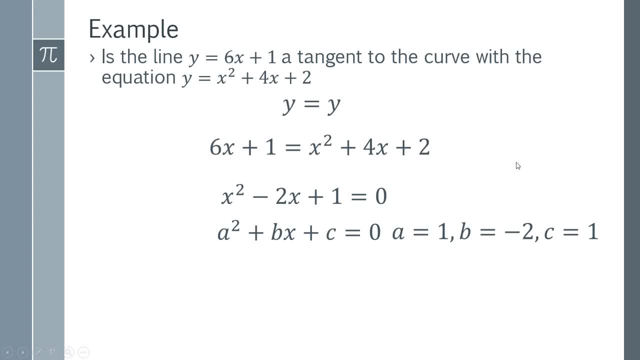 say that a is one, b is minus two, So we've got a plus one, so plus c is going to be plus one, So we've got a minus two and c is one. We then have our discriminant formula and we're predicting that if this is a tangent, so if this statement is true, that this line is in fact a tangent to that, 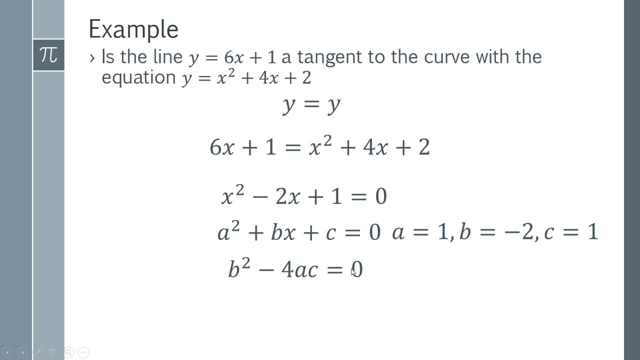 curve. we'll have the condition that this statement is true: that b squared minus four ac does equal zero. If it doesn't equal zero, then six x plus one is not a tangent to this line. So we substitute our values of a, b and c in like so, and you can see that minus two is a tangent to that curve. 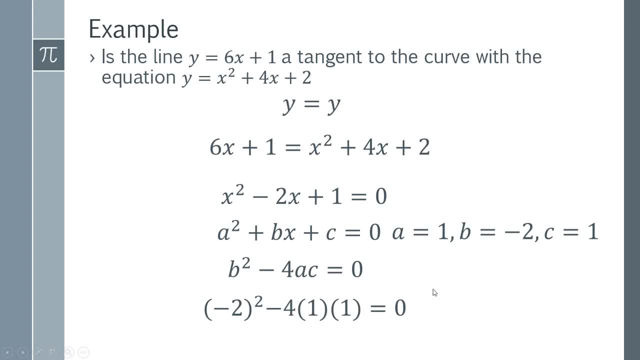 Minus two squared is four minus, and that's all going to multiply up to four, and so you get that zero equals zero, and therefore that has proved that this must be a tangent. So we kind of assumed that it was a tangent when we made this statement, and we've proved that that is in fact true. So